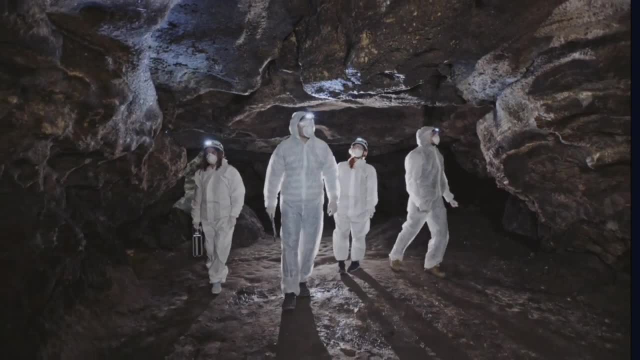 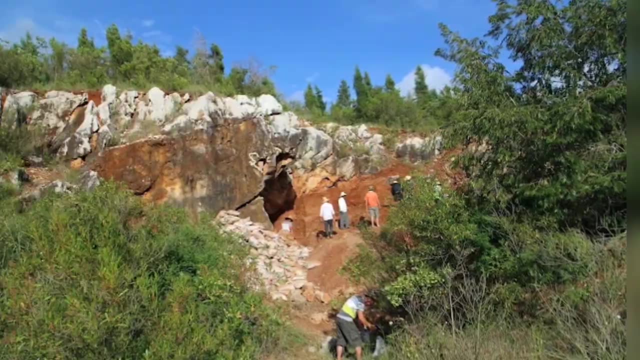 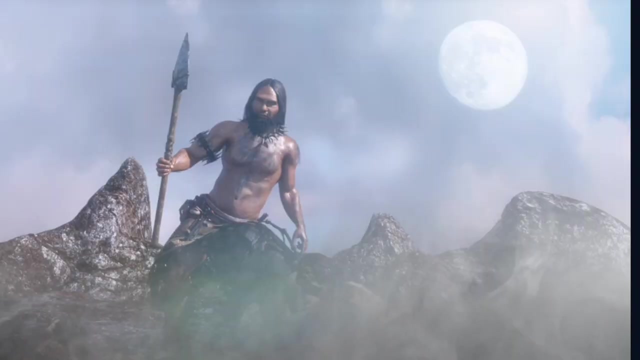 when a group of archaeologists in China discovered a large set of bones in the Maoludong, or Red Deer Cave in southern China's Yunnan Province. Carbon dating showed that the fossils were from the late Pleistocene, about 14,000 years ago, a period of time when modern humans had migrated to China. 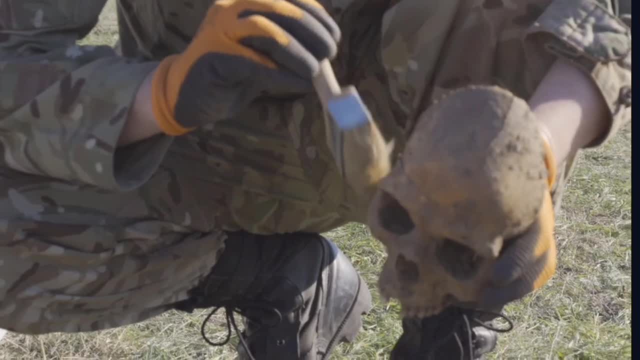 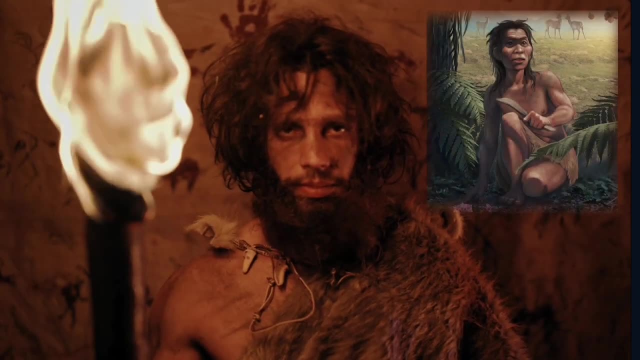 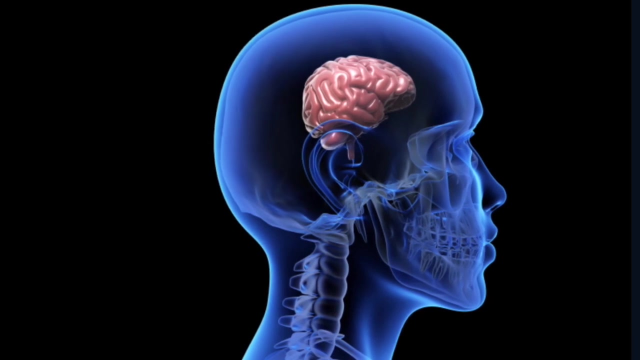 From the cave, researchers recovered a hominin skull cap with characteristics of both modern humans and archaic humans. For example, the shape of the skull resembled that of Neanderthals and its brain appeared to be smaller than that of modern humans. 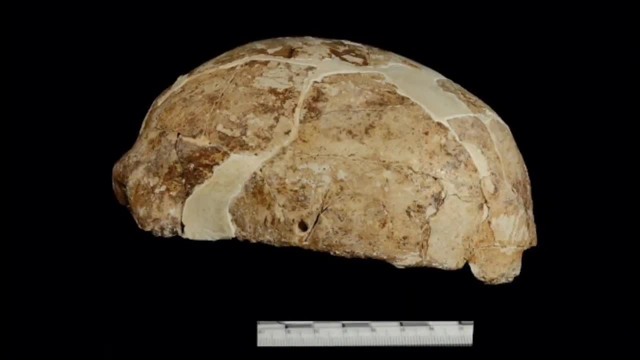 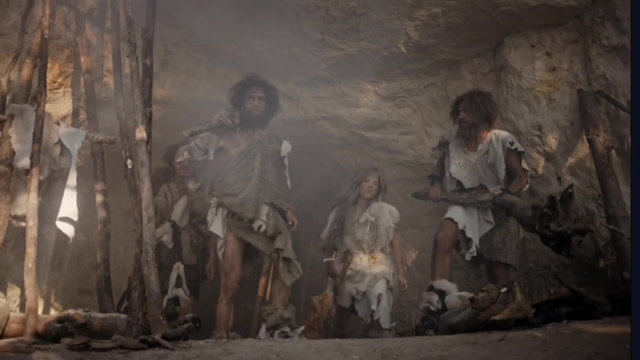 As a result, some anthropologists had thought the skull probably belonged to an unknown archaic human species that lived until fairly recently, or to a certain extent, in the Middle East. In 2018, in collaboration with Xiping Ji, an archaeologist at Yunnan Institute of Cultural 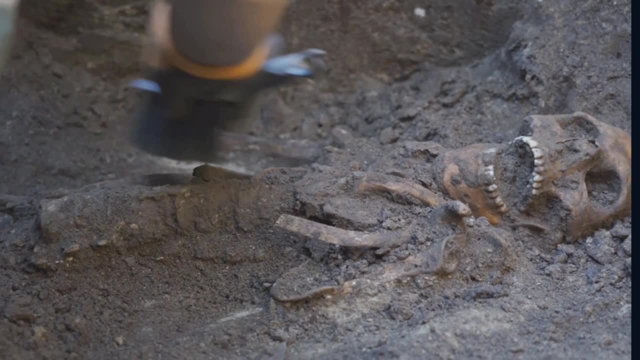 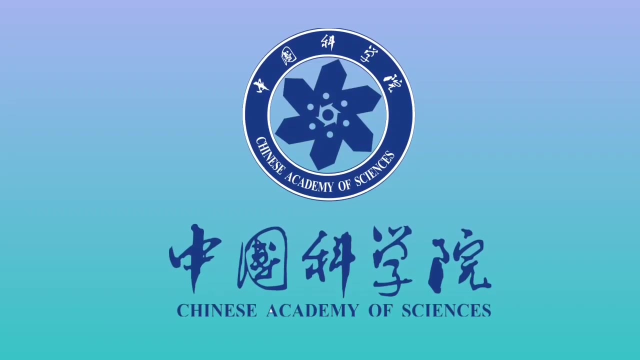 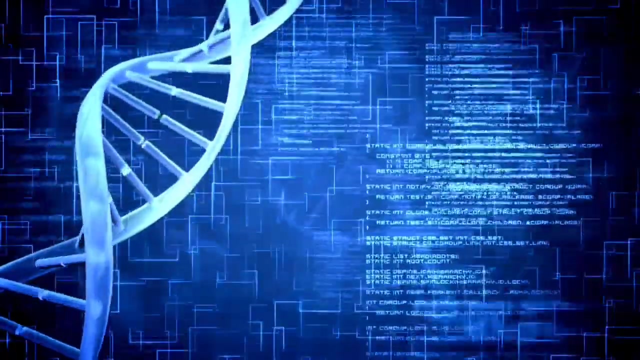 Relics and Archaeology, Bing Su at Cumming Institute of Zoology, Chinese Academy of Sciences, and his colleagues successfully extracted ancient DNA from the skull. Xinomic sequencing shows that the hominin belonged to an extinct maternal lineage of a group of modern 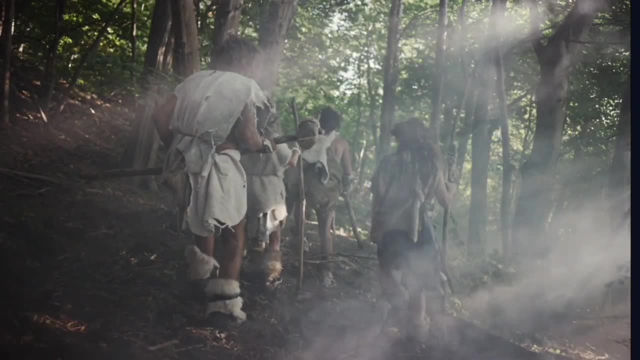 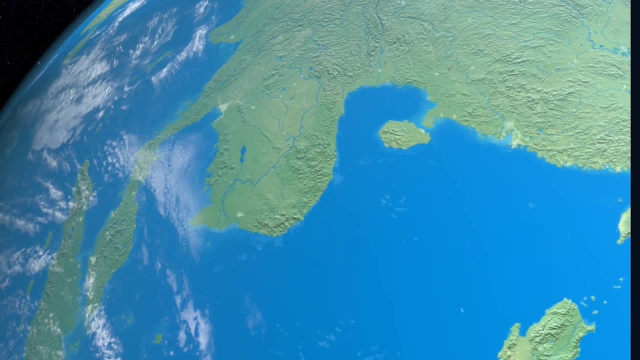 humans and that the skull was originally found in a cave in Yunnan Province. The skull is now found in the East Asia, the Indochina Peninsula and Southeast Asia Islands. The findings also show that during the late Pleistocene, hominins living in Southern East Asia. 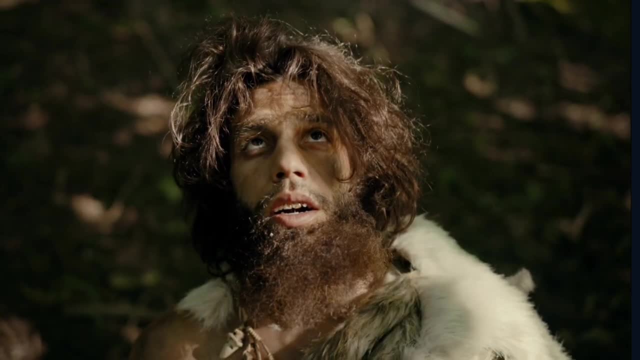 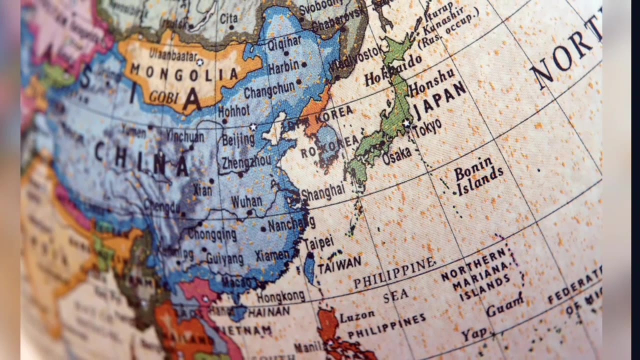 had rich genetic and morphologic diversity, the degree of which is greater than that in Northern East Asia during the same period. It suggests that early humans who first arrived in Eastern Asia had initially settled in the South and that the early humans had a lot more genetic. 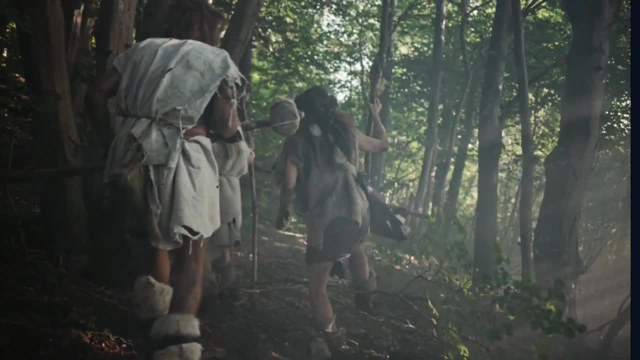 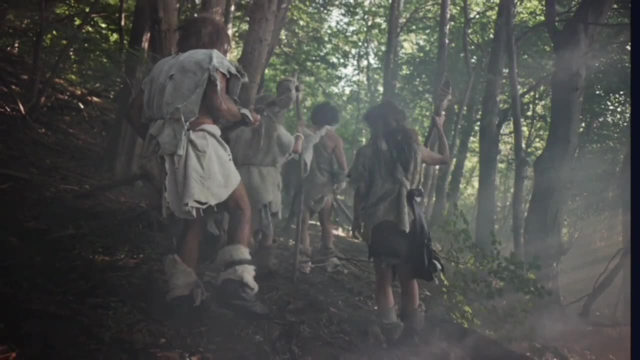 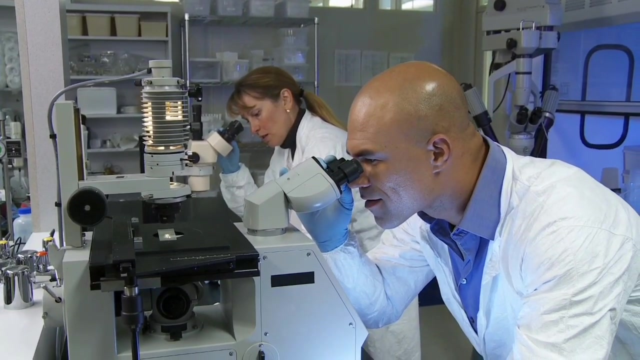 and morphological diversity than the early humans Before some of them moved to the North. Su says it's an important piece of evidence for understanding early human migration, he says. Next, the team plans to sequence more ancient human DNA by using fossils from Southern East Asia. 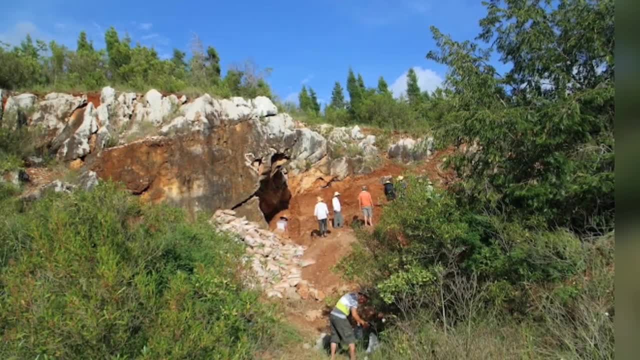 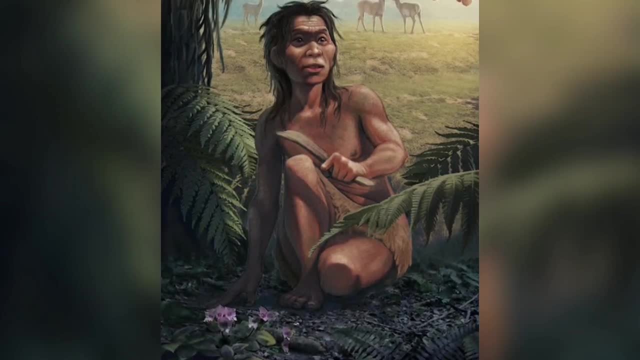 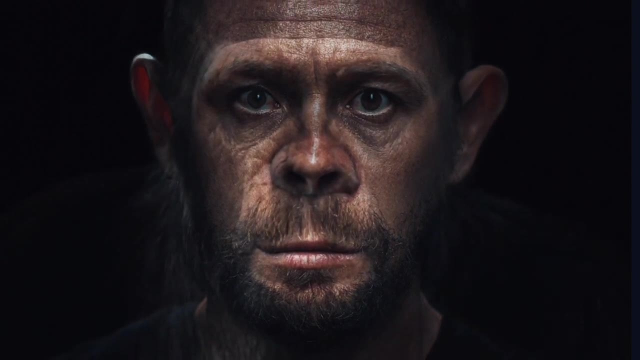 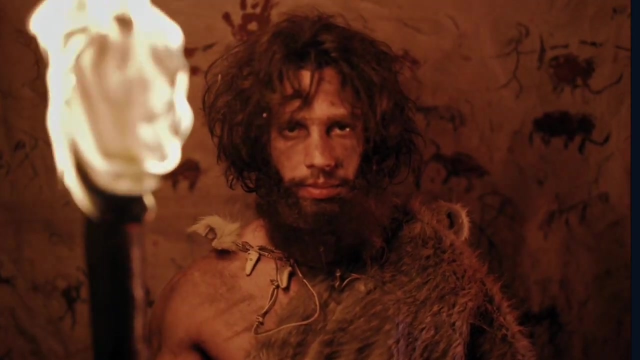 especially ones that predated the Red Deer cave people. Such data will not only help us paint a more complete picture of how our ancestors migrate, but also contain important information about how humans changed their physical appearance by adapting to local environments over time, such as the variations in skin color in response to changes in sunlight exposure. Su says: 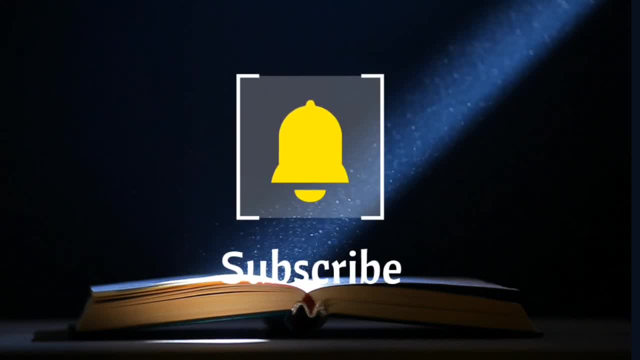 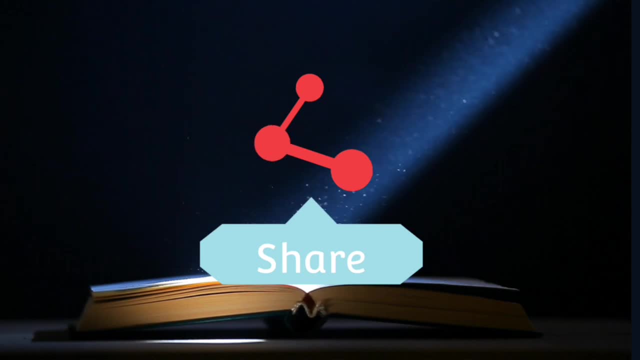 Next Let's take a look at a rough sketch of the first five Huns of the late Pleistocene period on s3.. In the original Huddle you can see that the late Huns were people who lived in the southern parts of the Great Ocean and the Silesian part of the Pacific Ocean itself. Their looks are more or less the same, which is the result of a similar fulfub insensitivity with the sicilian origin of the word, Dunstan, which is the southern part of the Pacific layouts and the east of the mountains of the island of Dunstan, and brings more of a sense of 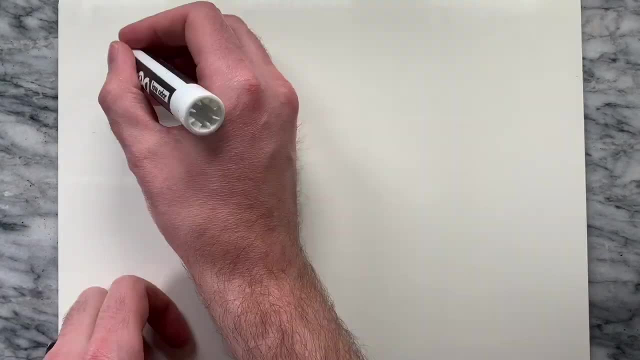 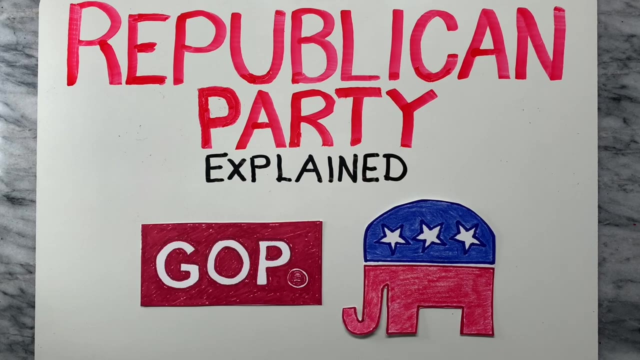 Hey, it's Dan Zimmerman. Welcome to Illustrate, to Educate. Don't forget to like and subscribe to support more simple and objective videos on topics that matter. In this video, we are going to take a look at the Republican Party platform to form a clearer picture of what they believe in. 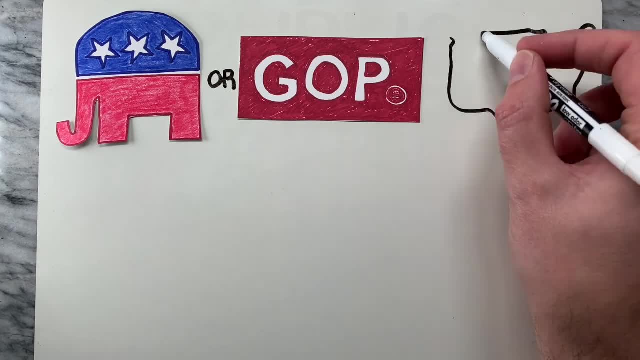 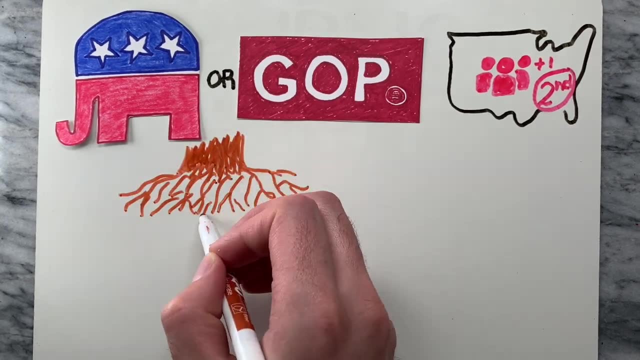 The Republican Party, also referred to as the GOP or Grand Old Party, is the second largest political party in the United States. The Republican Party's roots can be traced back to 1854, by antislavery activists who opposed the Kansas-Nebraska Act. which allowed for the potential expansion of slavery into the western territories. The Republican Party is generally based on American conservatism, contrasting with the modern liberalism of the Democratic Party, Republicans generally support supply-side economics. Some fiscal policies influenced by this theory were popularly known as Reaganomics. 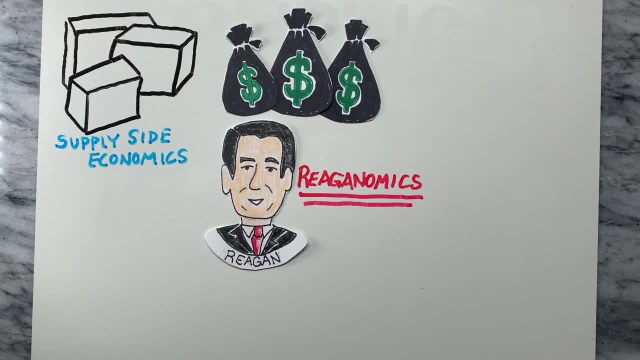 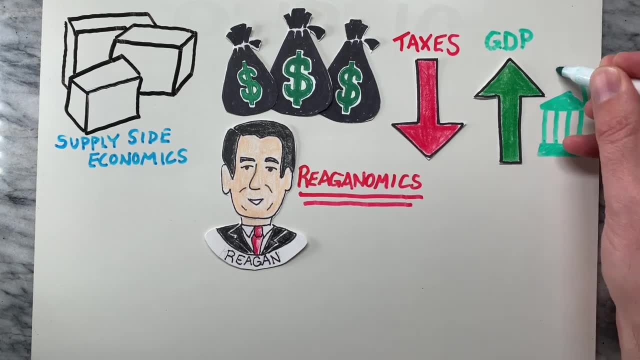 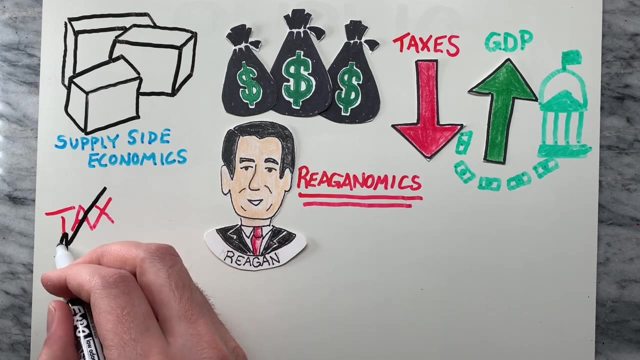 a term popularized when Republican Ronald Reagan was president. This theory holds that reduced income tax rates increase GDP growth and thereby generate the same or more revenue for the government from the smaller tax on the extra growth. This can be seen historically in the party's overall support for tax cuts. 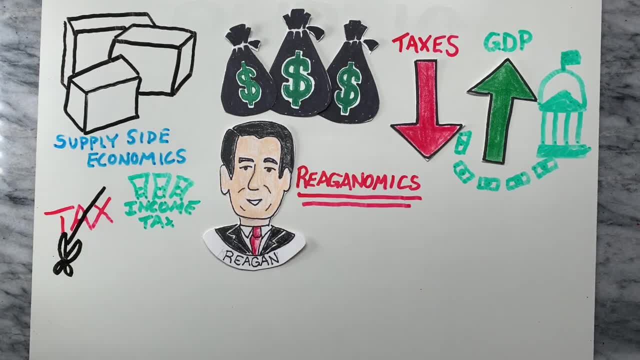 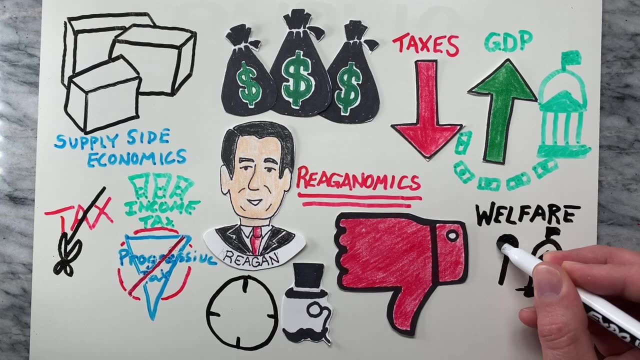 Many Republicans consider the income tax system to be inherently inefficient and oppose progressive tax rates, which they believe are unfairly targeted at those who create jobs and wealth. The Republican Party opposes government-run welfare programs for the poor, believing it encourages laziness and dependence on the government.